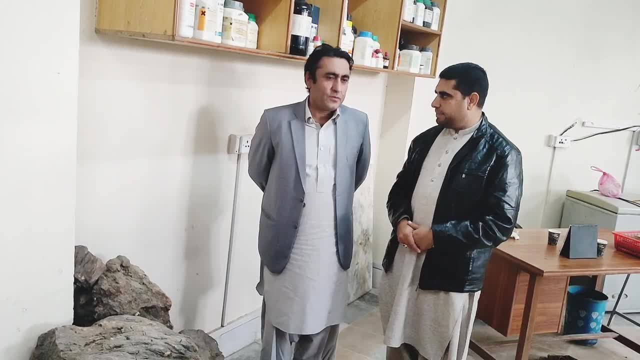 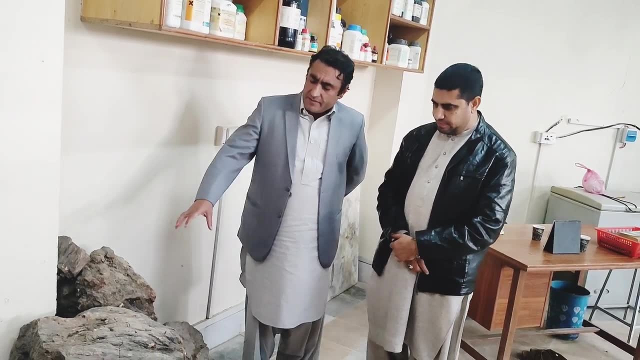 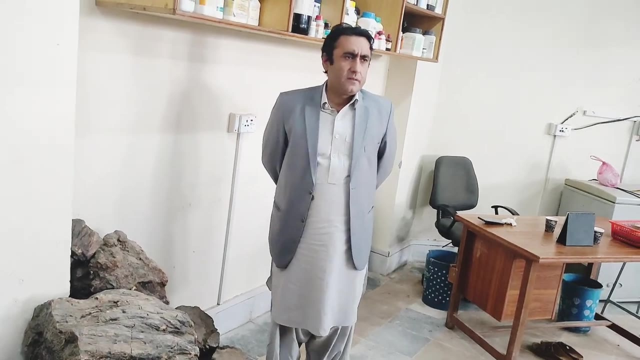 So Anand sir is with us and he is the chairman of the department of botany. So, Anand sir is We always welcome you for visiting, again and again, and this time, actually, these fossils. they have been collected from the Badakhil area, which is approximately 20 to 30 kilometers. 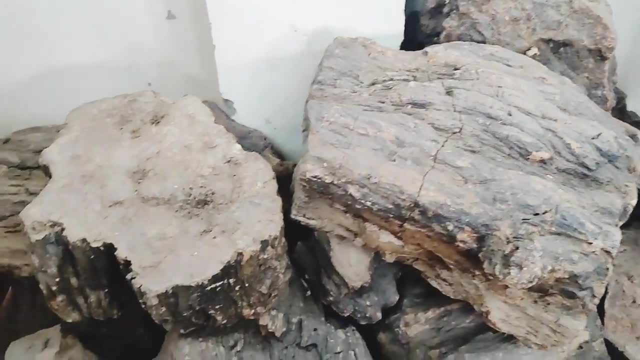 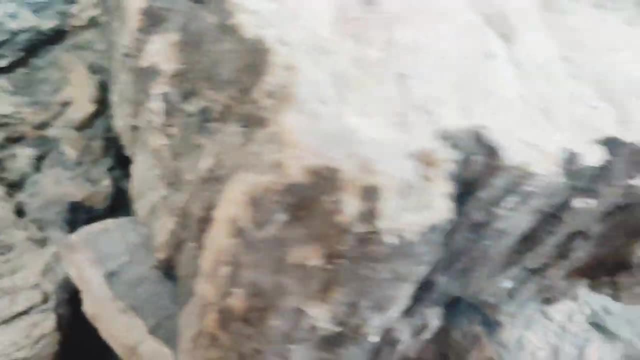 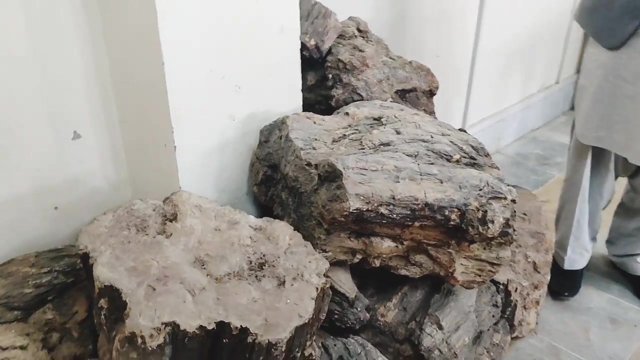 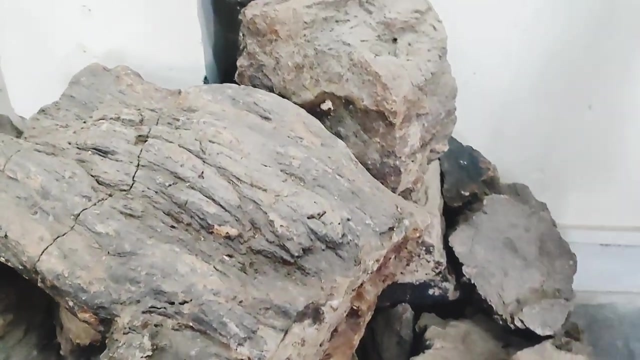 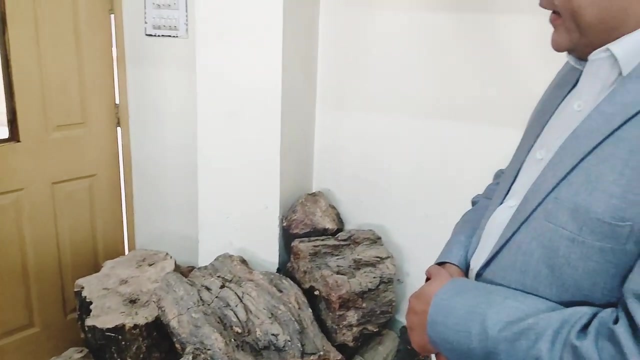 from here and basically this whole area, I mean the proximity of district Kohat. they have the potential of periobotany because there are certain more areas in which there are some types of fishes as well as plants being fossilized. So the main idea behind this was to promote actually this field. and well, we are currently. 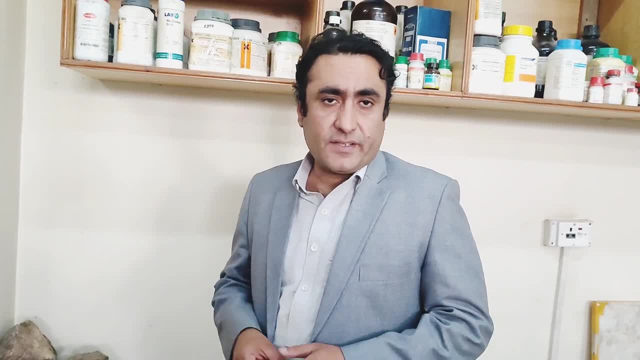 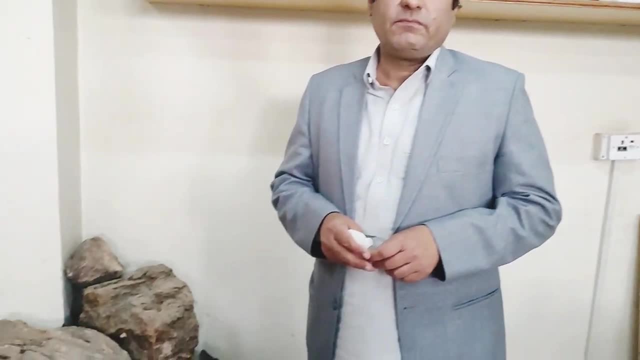 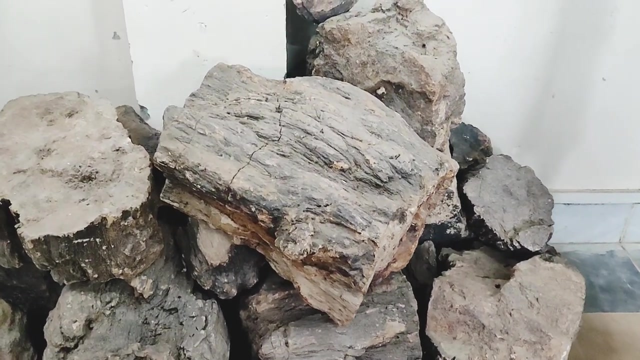 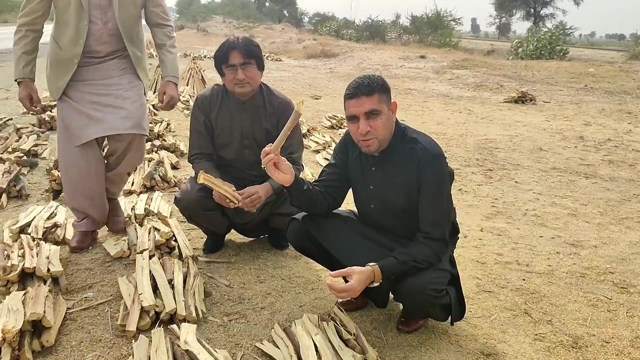 actually working on the identification of these fossils as well. So, yes, it's an emerging field, particularly in Pakistan and abroad. of course, many modern research and applied research is currently being carried on these fossil plants. Here you see, these are the small woods that are collected from the stem of Prasupas celeraria. 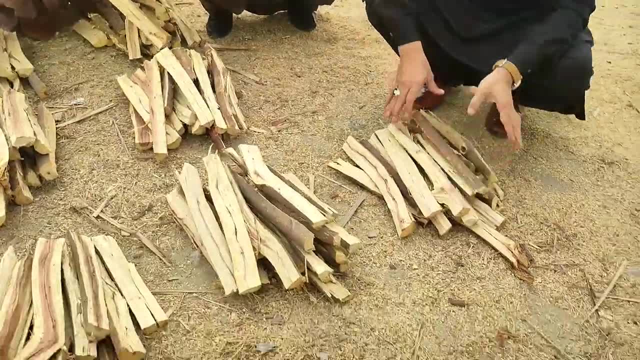 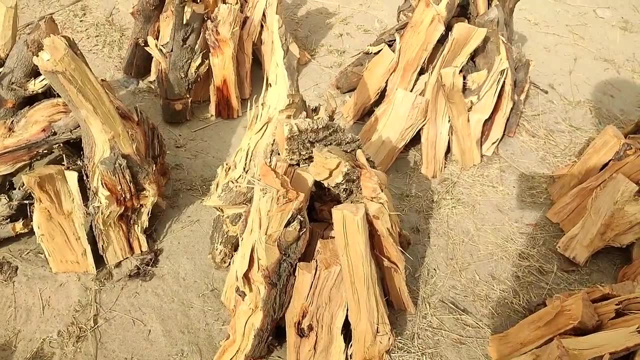 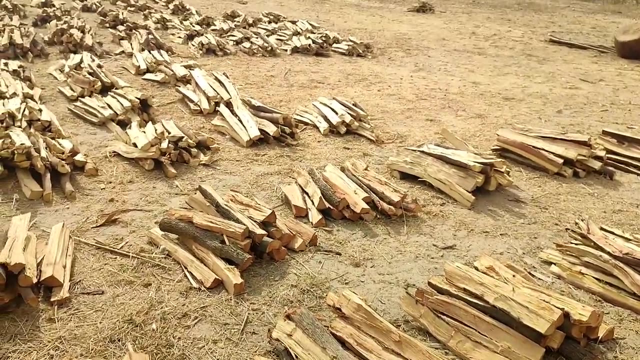 Prasupas, judiflora and Acacia modesta. These woods are used in deforestation. These are the surrounding areas for making the stoves, and they are used for stove heating during the winter season. So this is the traditional way to warm up the rooms for winter season and to avoid from 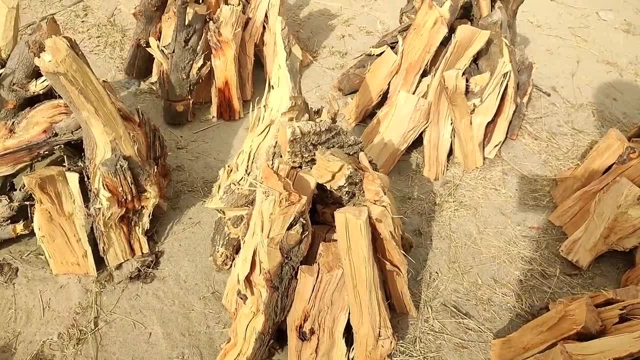 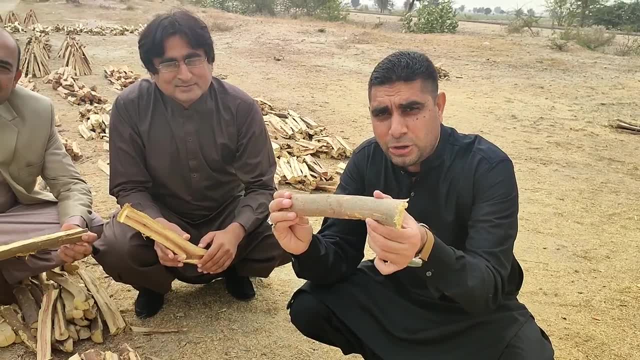 the coldness. they use these small woods for heating purposes. So this is an additional of the woody plant that is, Prasupas celeraria, Prasupas judiflora and Acacia modesta. Thank you.